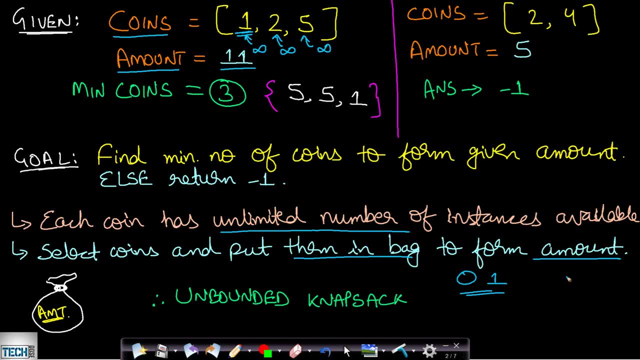 similar to the 0- 1 knapsack. there we can have one instance, exactly one instance of each item. and then we were having a bag where we were picking up the items and putting it inside a bag. here also we are having the bag which is of capacity amount. 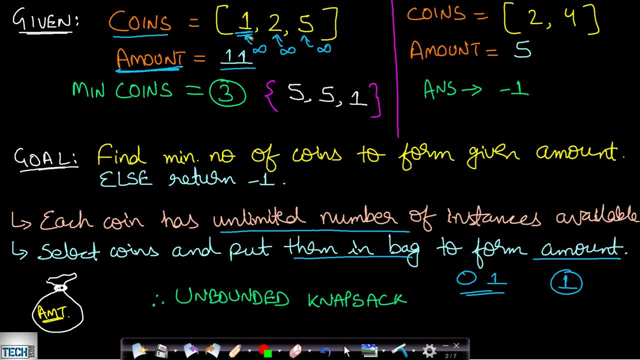 we want to fill, but we want to fill it with the coins, and each denomination of the coin can have infinite number of instances. so this is not just bounded to, let's say, one instance, but it is bounded by infinity. that means it is unbounded, okay. so that is why this problem falls under this unbounded. 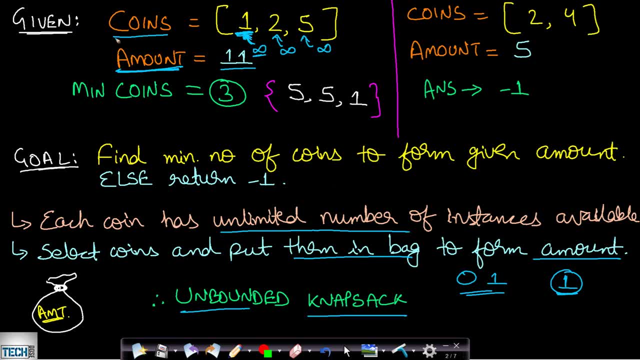 knapsack problem. now let us look at this first example, where we are given the coins array and we are having three denominations- one, two and five- and our amount to be formed is 11.. there are many possibilities which we can take in order to form this amount. like we can take 11 ones and still we 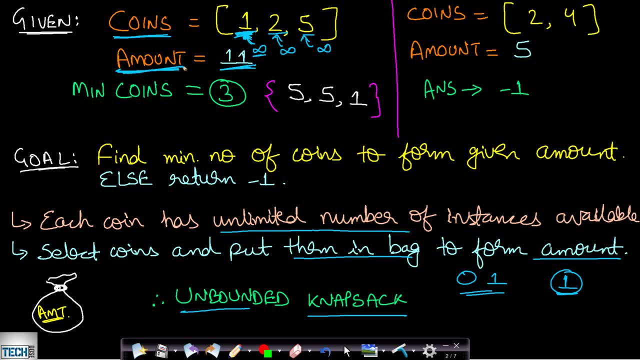 get this 11.. but we want to form this amount using minimum number of coins. so here the minimum number of coins will be equals to 3 and the distribution will be: we can take two number of fives and then one number of one, okay, so these three coins together will be making this amount. so 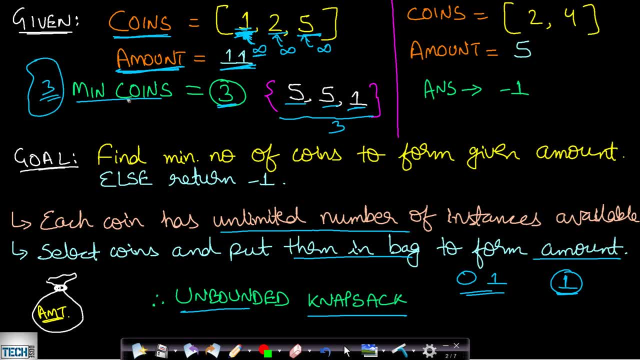 inside the bag. the minimum number of coins we need is three. therefore, we will return three coins as our answer. now let us look at the second example, where we have coins as 2 and 4 and our given amount is 5. now here we will not be able to make this amount 5, even if we include any number. 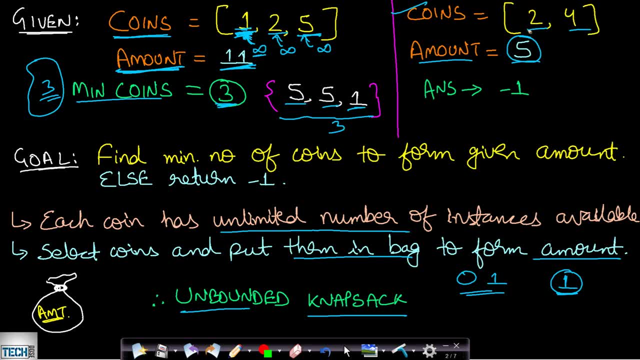 of instances of any denomination. so we can include two number of twos, but still we cannot form 5. so 5 is impossible to be formed, and so we will return minus 1 in this case, saying that this amount can never be formed from the given denomination of coins. so this is the entire. 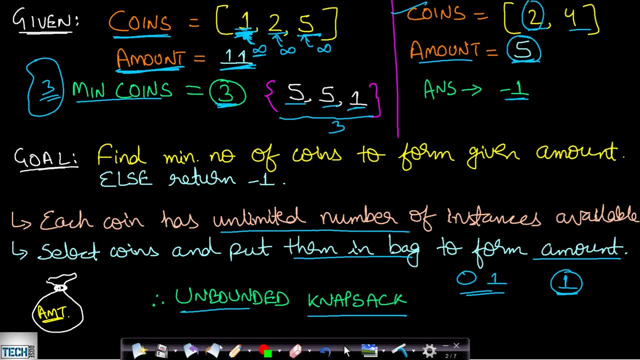 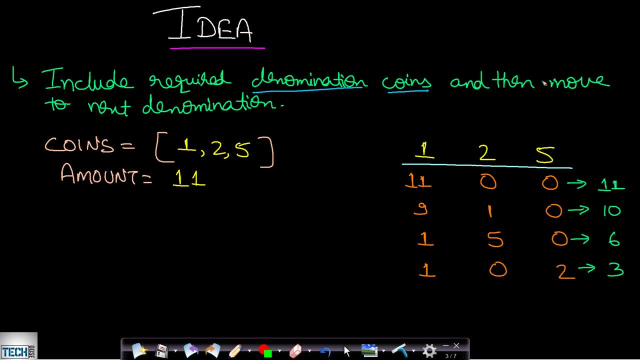 problem and i hope you were able to understand it. now let us see an idea behind solving this problem. we need to include the required denomination coins and then we move to the next denomination. so one idea can be: we can take each denomination one by one. let's assume that we are taking 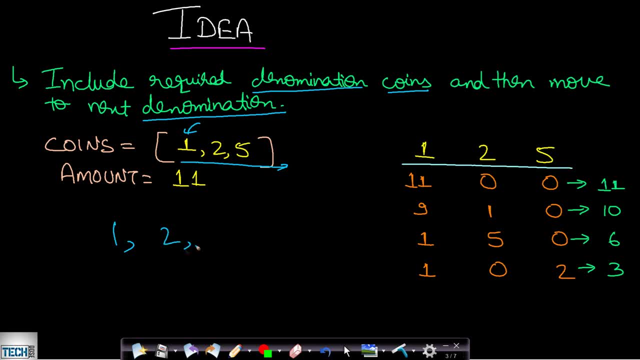 denominations from left to right. so when you have coins, let's say 1, 2 and 5, then you can take all the possible number of instances which you want to take for this denomination and then you can move on to the next denomination. when you move to the next denomination then you cannot come back and again make 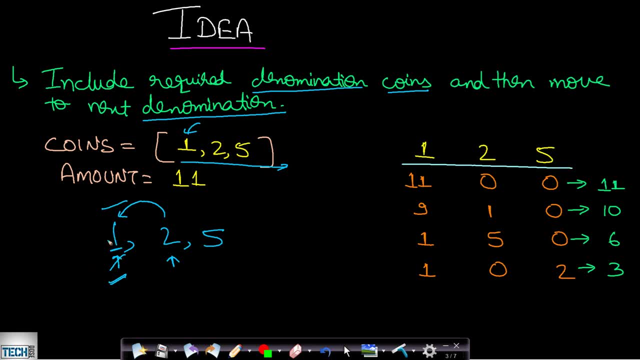 a choice for a given denomination. okay, so that is not possible. now, this is the assumption we are making. so let us say that we are taking the same example: coin says 1 to 5 and amount is equals to 11. so if we start from left to right, 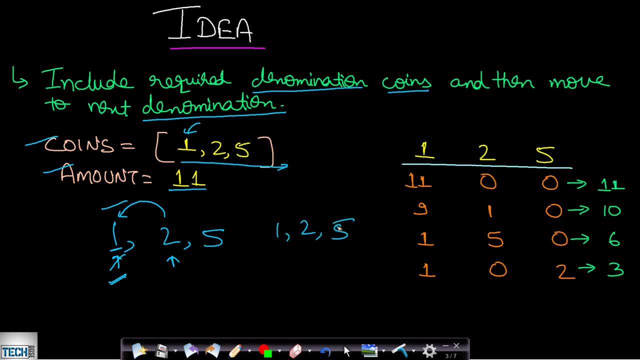 okay. so if our coins are 1, 2 & 5 and if we start from this 1, then we can take this 1 any number of times, but we should not exceed this amount. so we can take 1 11 number of times and we can move to 2 and we can include 2- zero number of. 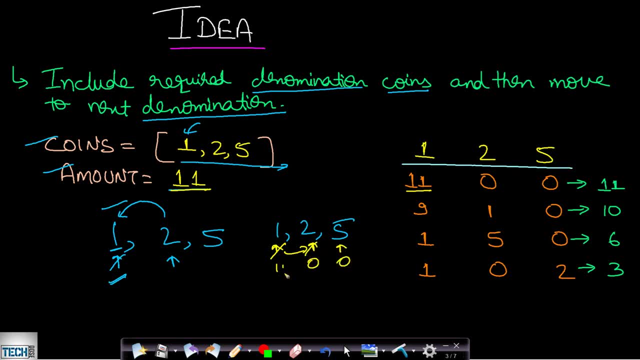 times 5- zero number of times- and still we can make amount equals to 11. okay, but in this case, even if it was possible to form a mount, that number of points which we consumed was equals to 11. let us see some other possibilities. so for this one, 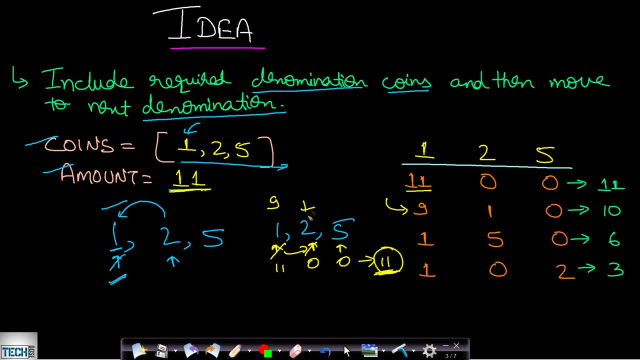 we can take 9 number of points and then we move to this 2. we can include one instance of this 2, we can move to 5 and so on. okay, so here also we are making use of 10 coins, and if we try other possibilities, then 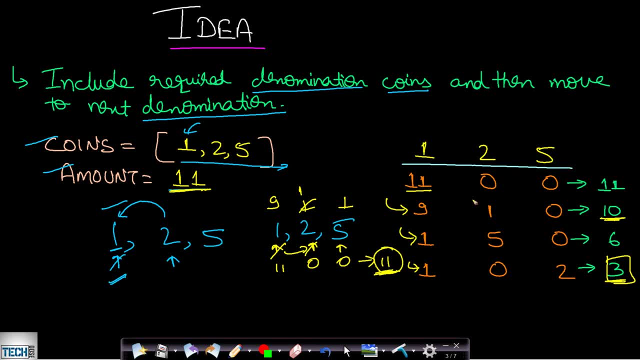 we will get the minimum as 3 number of points, which will be by including 1, one, one, zero, two and two number of fives. so this is the best possible combination. okay, i hope you are understanding it. in this problem, we will be moving from left to right while making our decision. 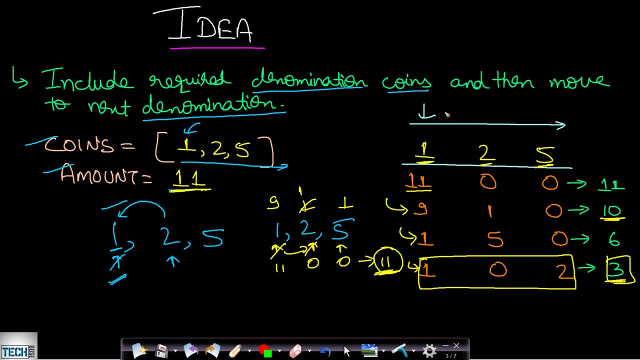 so once we are at this first coin, we can take any number of instances, but once we move to the next coin, we cannot come back to this coin and make other decisions. okay, that is not possible. so this is the assumption which we are making in solving this problem by using recursion. okay, so we will. 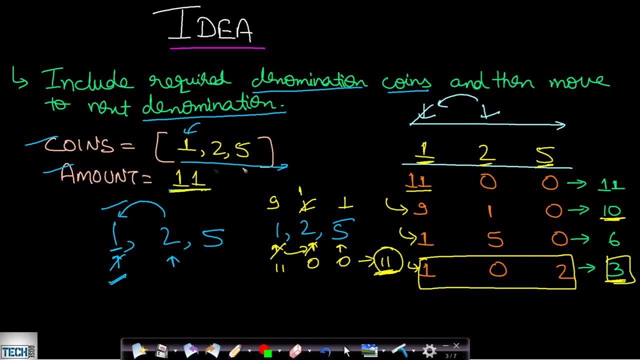 not be solving it just randomly now here. as i had already told you, one will be having two choices, and we can make two choices, that is, either to include it or exclude it any number of times. we can make these choices any number of times and then we will move to the next denomination. 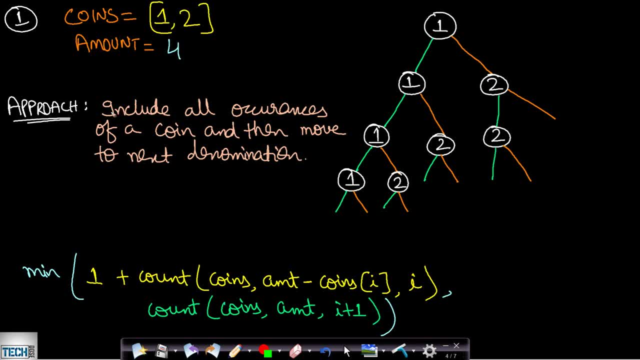 so that is the idea. so our idea is to include all the occurrences of a coin and then move to the next denomination. so i will take the similar example. like coins will be one comma two and amount of coins will be one comma two and amount of coins will be one comma two and amount of coins. 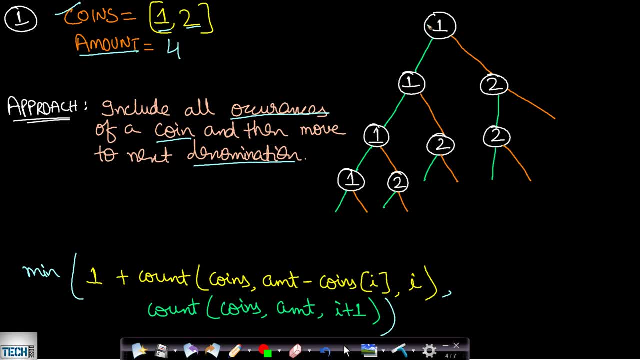 to be found will be four. so if we draw a tree diagram, then if we are at this first denomination, we were having two coins. we are at this first denomination, one. now if we include this one, our amount to be found was four. if we include this one, it will be three. if we again include 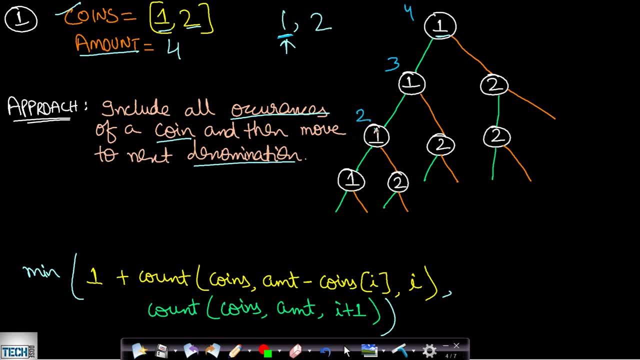 this one, our amount to be found will be two again. if we include this, one amount to be found will be one again. if we include this, one amount to be found will be zero and the total number of coins here will be equals to four. okay, if we exclude this one, then our amount to be formed 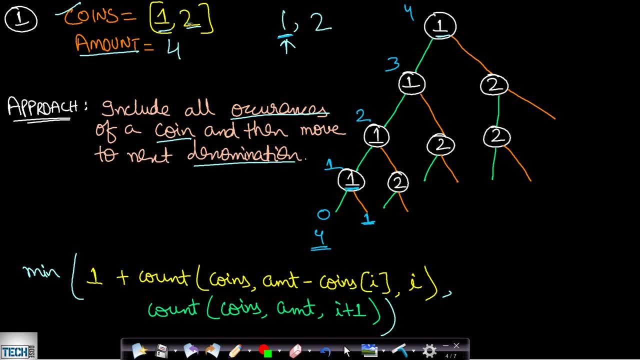 here will be one and now we will be having the next denomination, which is two. so if we are having denomination two and amount to be found is one, it will not be possible to form either we exclude it or include it. so this will not be possible. therefore, we will backtrack now. we will backtrack. 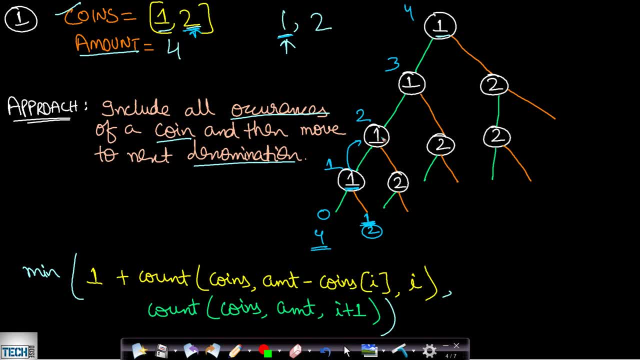 to this one. now here we had included this one, but if we exclude this one we will have two denomination. so if we exclude this one, then amount to be formed here will be two, and since the next denomination after excluding this one, we cannot go back and include it if we are at this two. that means this: 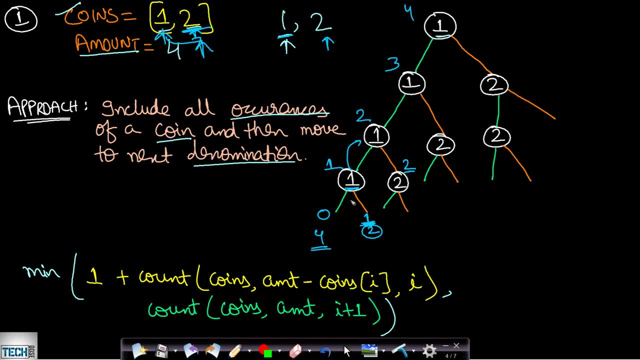 two, then we can include this two in order to get our required amount, because amount to be formed here is two. we can include it and then the number of points will be one. one, one, one, and then this one was excluded, so total coins will be three. so earlier we had used four coins to form this sum. 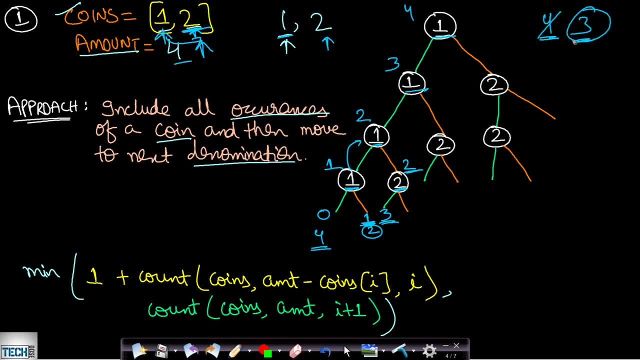 we are having three coins, so three is better, which is minimum. so we will be taking the minimum number of points and, like that, we will pass through the entire tree using recursion and find out the minimum number of coins to form this amount. if there is no combination in order to form this, 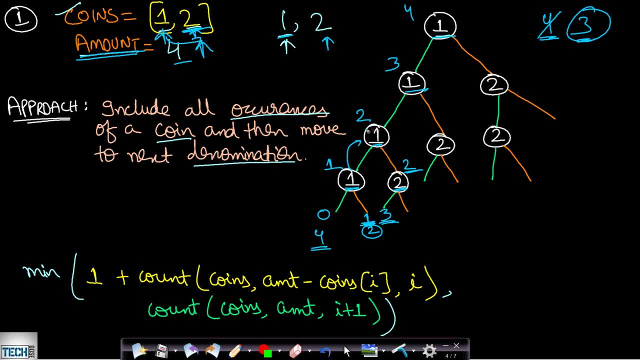 amount, then we will simply return minus one. now we can write the recursive code by using this formulation, like if we are including a given denomination- let's say we were at this one- and we can των in the value of the value of this amount. this is the value that we want to keeping. 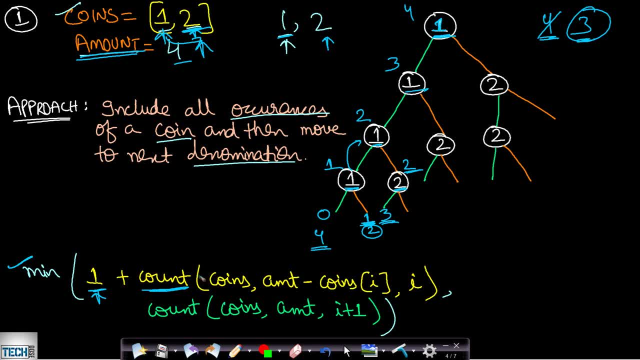 in the bag will increase by value one and since we are including this one again, we can include this same coin. therefore, this is our coins array, this is our amount. if we are including the current item, which is the ith element, then coin set, i will be decreasing this value amount because initially we 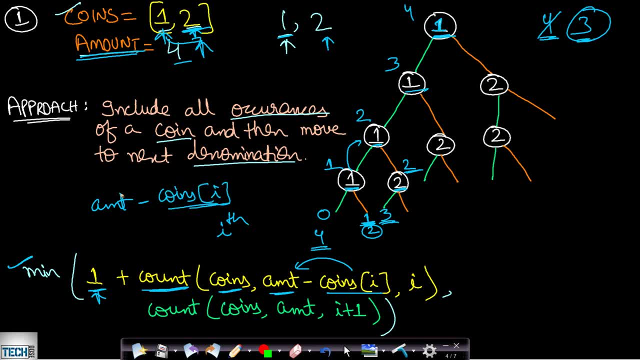 were having amount and now, since we are including the ith coin, then the ith coin value will get decremented from the total amount to be formed. okay, so this is our coins array. this is the new amount after including the i-th element, and this is the i-th element when we are including a coin. we will continue to stay at that denomination. 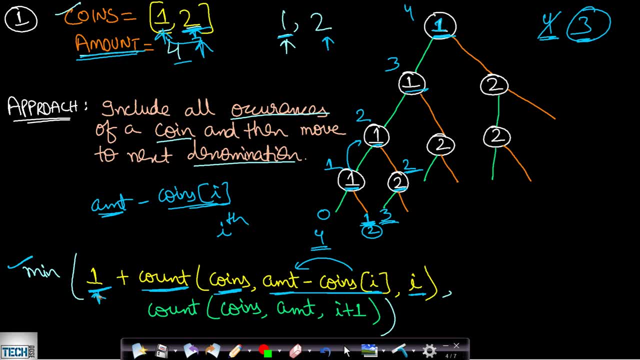 and try to include as many as we can or as many as we want, which will give us the optimal answer. okay, we do not initially know the optimal answer. we will have to try all possibilities. so this is for the inclusion case. if we have decided not to include this denomination, then we will move on to 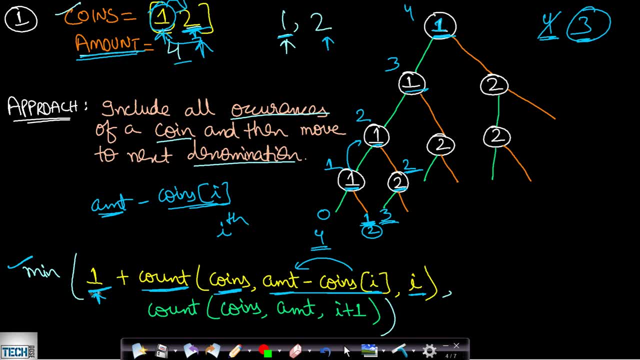 the next denomination, and so our number of coins will not increase and we will be passing the coins array. our amount will remain the same and we will be moving to the next denomination, which is i plus one-eighth denomination. this is how we can write the recursive code. i hope you understood this. 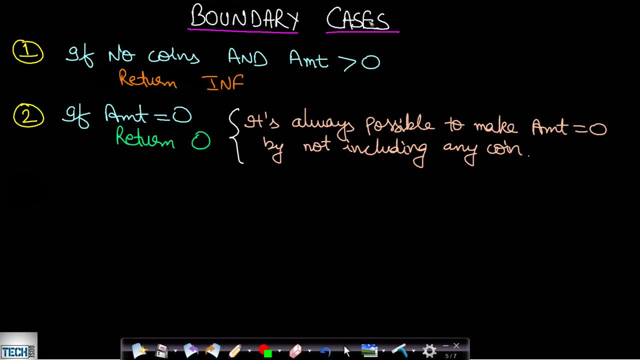 formulation now, the boundary cases in this problem are: if we are having no coins and if the amount to be formed is greater than zero, then obviously it will not be possible to move on to the next denomination because we are having no coins and we will return infinity in this case. otherwise, if the amount to be 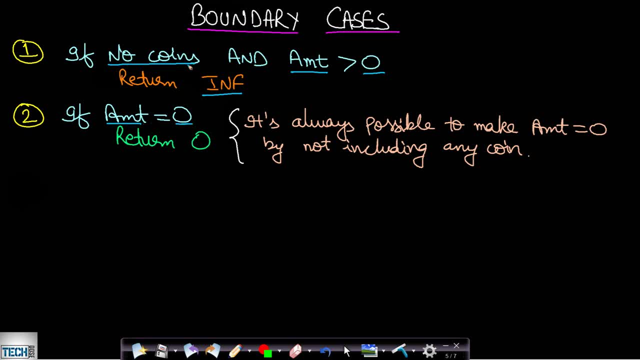 formed is equals to zero, then no matter if we are having any coin or not, it will always be possible to form an amount equals to zero by not including any coin. and if we are not including any coin, then the number of coins will be zero. therefore, it is always possible to make amount equals to zero. 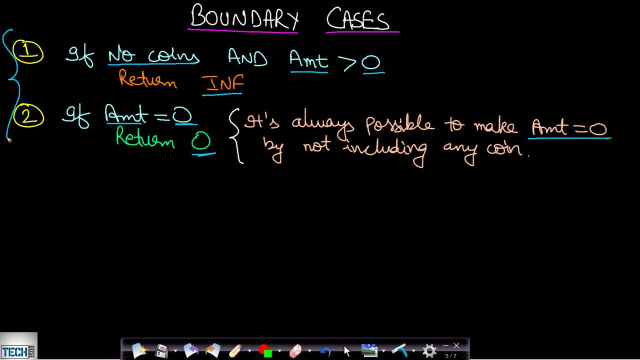 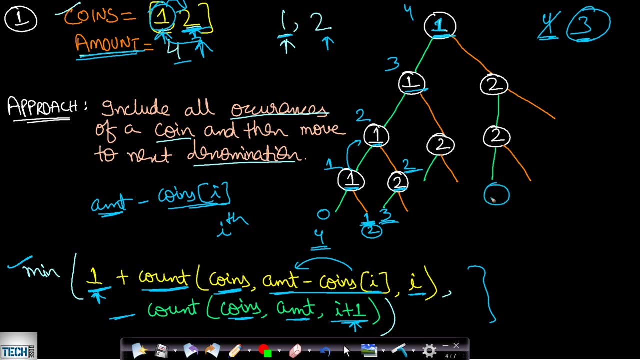 by not including any coin. so these are the two boundary cases for this problem. now, in this problem there will be optimal substructure. that means solving a smaller sub problem and using it can solve the bigger sub problems, and there will be repeating sub problems if you take some larger examples. okay, so since we will be having both those properties, we can. 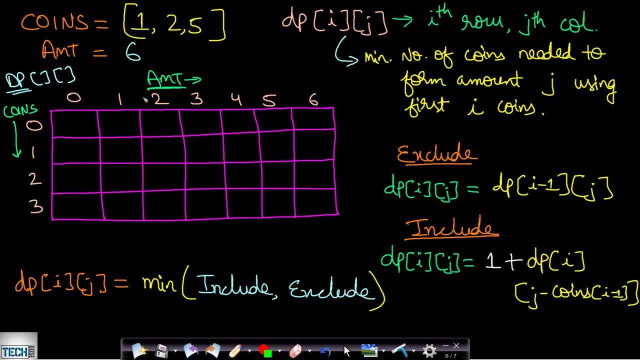 use dynamic programming in this case. so let us see the tabulation dp and let us understand how to use it in order to solve this problem. now we are having, let's say, three number of coins- one, two and five- and our amount to be found will be six. now i am taking the columns to be equals to amount. okay, so 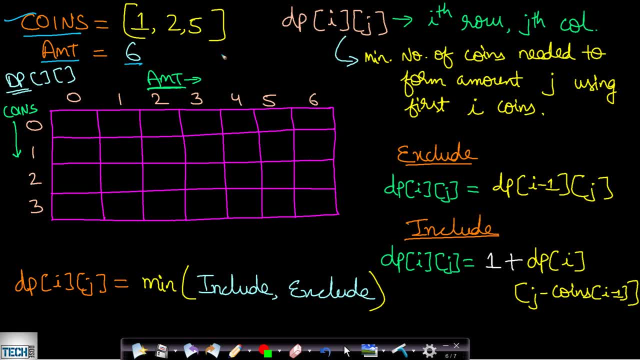 this dp table will be of size, number of coins plus one, that is n plus one, and amount plus one, that is m plus one. and we are taking one extra size because we want to consider these boundary cases which i had explained here. now, if you consider the boundary cases, then if we are having no coins and if the 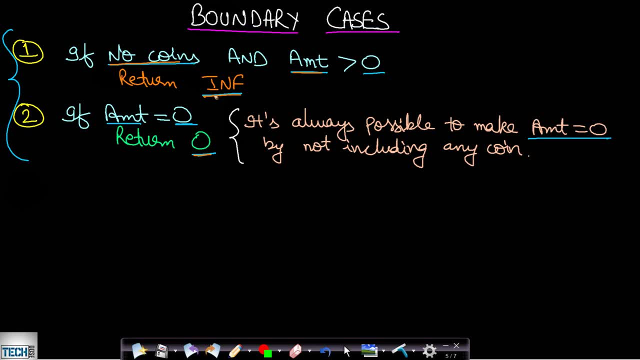 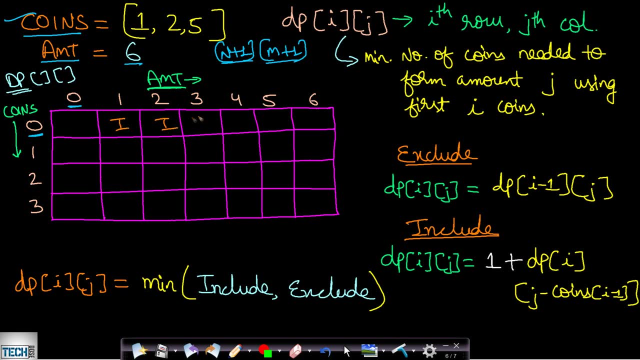 number of coins is greater than zero, then it will not be possible to form this amount, and so we will be returning infinity. so, for these all values, we will be having infinity because we are having no coins, we are having zero number of coins and the amount to be formed is greater than zero. so it 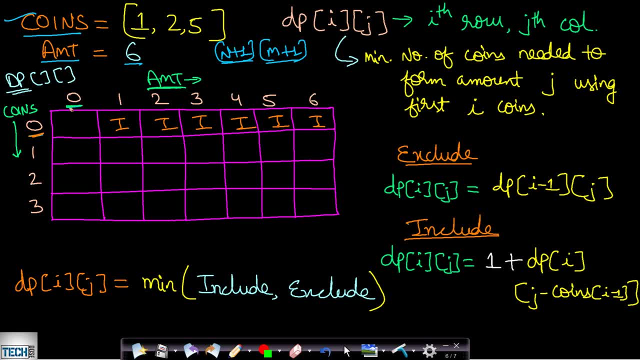 will not be possible. and for the other case, if we are having amount to be formed as zero, then it will always be possible to form amount equals to zero by not including any coins. therefore, the minimum number of points in this case will be zero. okay, so this is how the first row and the first column 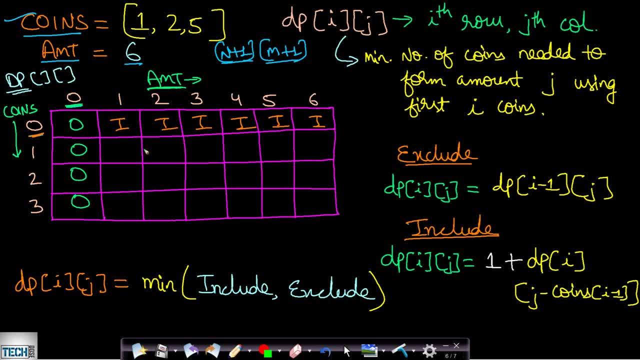 can be filled. now we will be filling the rest of the cells. so how do we do it? this is basically the sub problem. now, what is the sub problem in this case? if we are considering dp at ij, this table name is dp. we have taken coins on the row side and we have taken the amount on the column side. 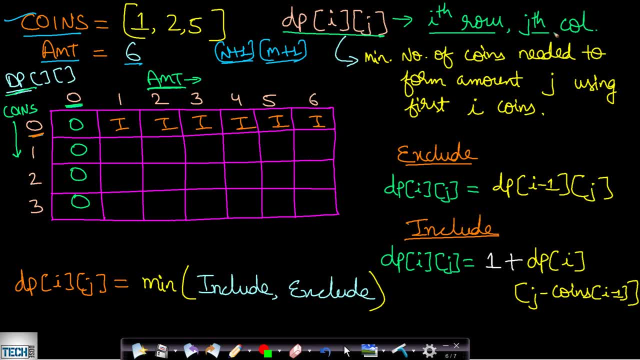 so dp at ij will mean that we are in the i th row and the jth column. now that will indicate the minimum number of coins needed to form amount j using the first i coins. so let us take this case. okay, so let us take this dp at 2 and at 3. what does this mean? 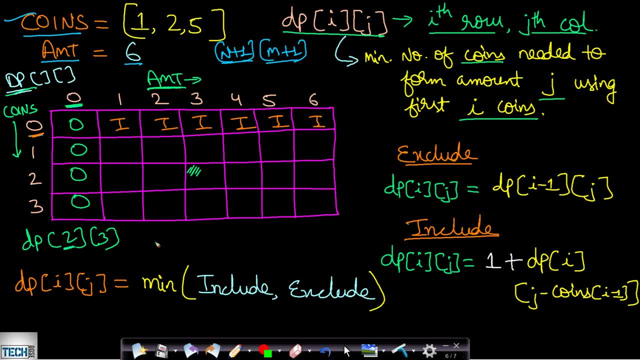 this means that if we are having the first two coins, that means if our coin includes 1 comma 2 and if the amount to be formed is equals to 3, then what will be the minimum number of coins in order to form this amount? 3, using coin denominations 1 comma 2, and each denomination can have infinite. 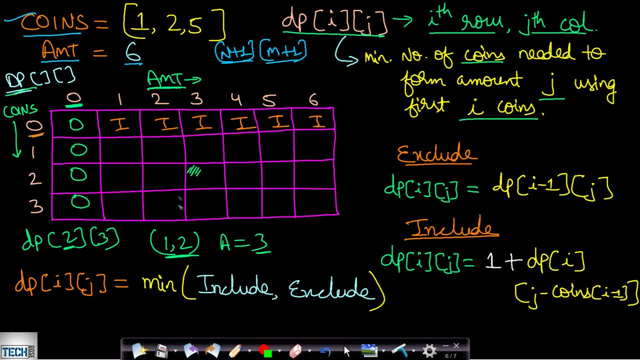 number of, uh, these instances. okay, so in this case, you can see that you can use one, two and then one, one. so you can use two plus one, which will form an amount equals to three, and the total number of coins will be two. so we will be filling two here, okay, so this is a sub problem and like this we. 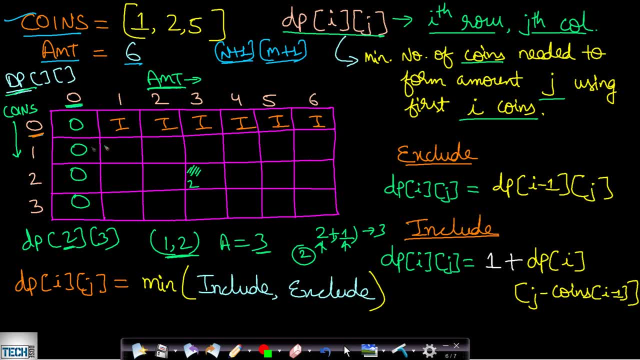 will be filling all the cells, so let us first start with this cell. one comma one. now here. one means we are having just the first coin. we are not having these two coins, we are just having this one. so if we are having coin one, then is it possible to form this amount one? yes, it will be possible by using one coin. 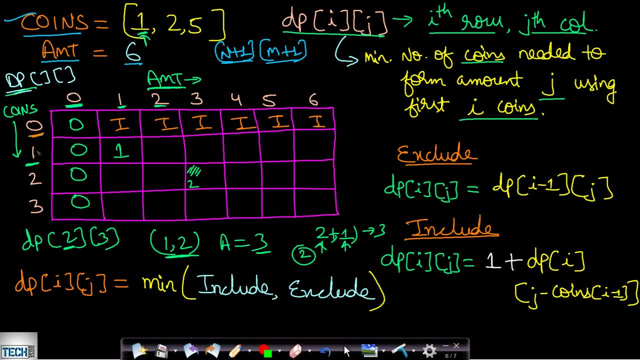 now, if we are having amount two, will it be possible to form this sum one? well, in this case we are having two choices: we can either include this coin one or we can exclude it. so if we are excluding it, then we will be basically seeing this value because we are 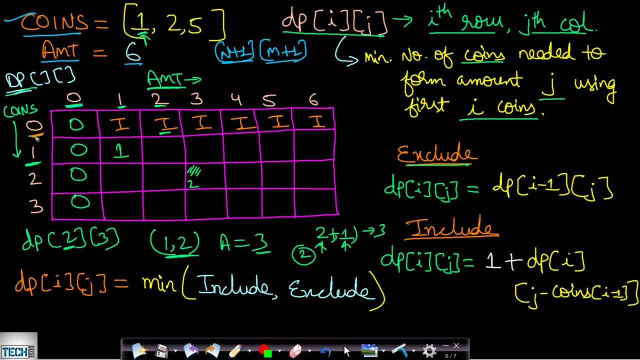 excluding this denomination entirely. so we will have one less number of denominations and then we will be forming the same amount. so if we are excluding this denomination, then dp at ij will be equals to dp at i minus 1, j. this i minus 1 is indicating one less number of denominations. 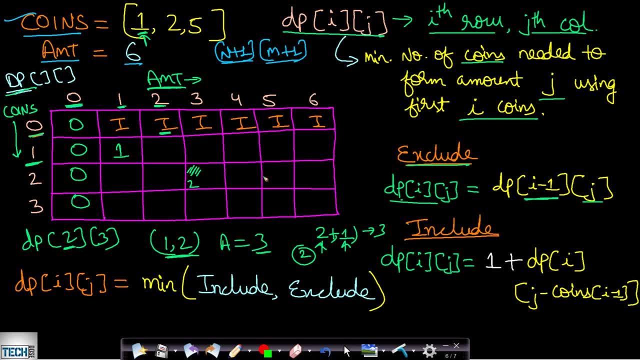 and if we are including this coin 1, then including means what we are including: this denomination, one instance of this denomination. therefore, the number of coins included in the knapsack bag will increase by one, and also the value which we have included will get added, and so the total amount to be formed. 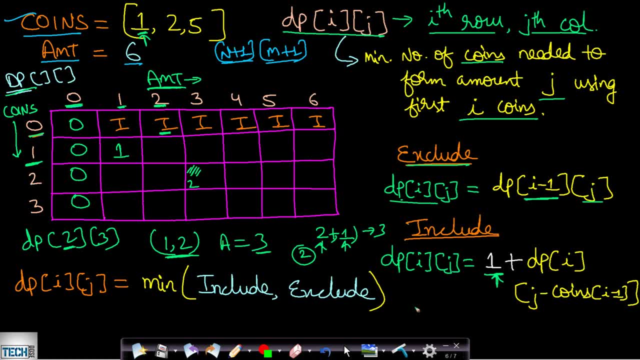 which is 2, will now get decremented, so it will become 2 minus the coin denomination size. so the coin denomination size is 1 here. so 2 minus 1 will be 1. therefore this y j here will be equal to number of coins which we have used, 1 plus dp at i. 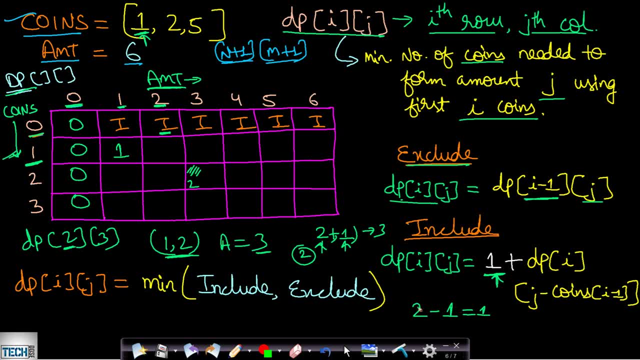 which is the same denomination, because if we are including a coin, then we can include some more number of points of the same denomination. that is why we will remain at the same row and then we will move the number of columns to the left by the amount of the coin. 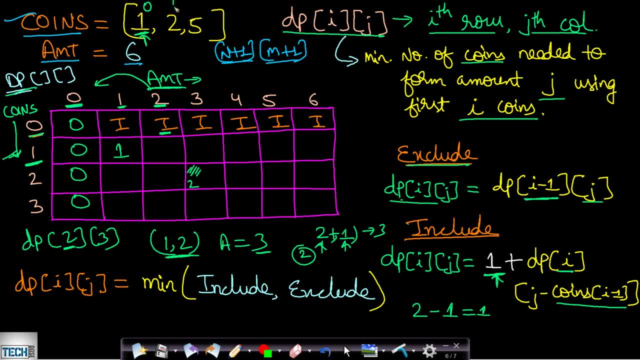 amount of the current coin included. okay, so here, as you can see, the coins array is actually indexed from 0, indexed from 0, zero, but the coins here will be indexed from one. one means the first coin, two means the second coin. okay, so that is why i have written here: i minus one, so we will be taking the minimum of. 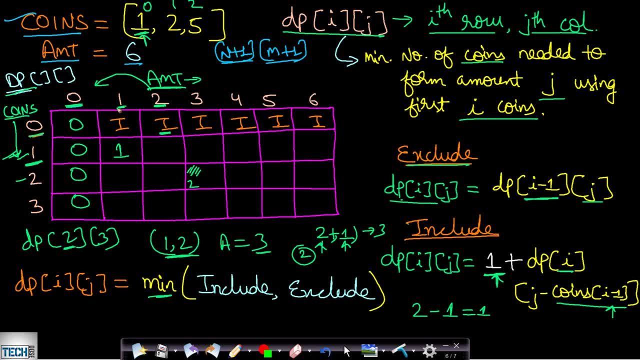 include, comma exclude. so if we are including this, then that will be equals to zero plus one, this one, and then, if we are excluding it, then that will be infinity. so what is minimum? one will be minimum, so we will be putting one here. okay, i hope you are understanding it. now let us say if we want. 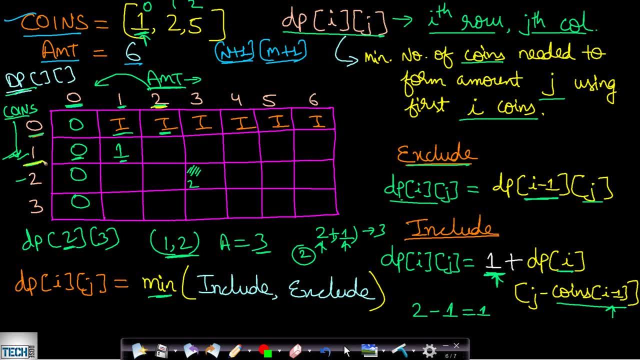 to form. this amount equals to two and we are having just the first denomination. if we include this first denomination, then its amount is one. now, if we include this one, then that will be one plus dp at i minus j, minus coins, at i minus one. so this one, one plus one, will be two. so minimum of 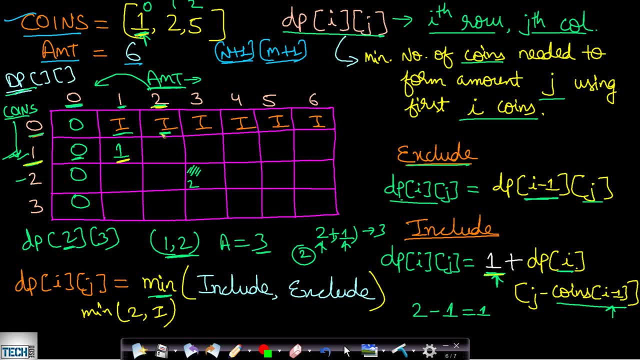 two comma infinity. what will be that? this infinity is coming from the exclusion case, so that will be equal to 2. so we will be writing 2 here. similarly for this, 3, it will come as 3. this will be 4. this will be 5. 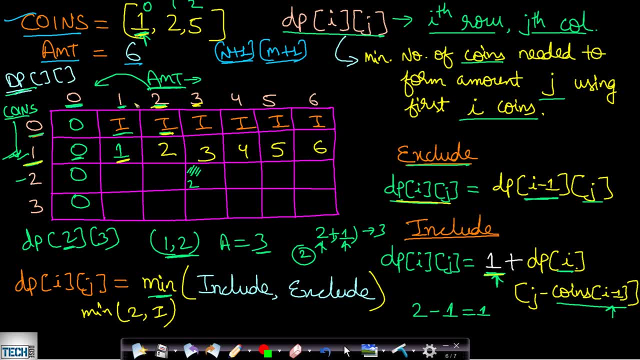 and this will be 6, so it is possible to form all these amounts. okay, now let us include the first two denominations. that means, if we are having this 1 comma 2, both, then what will be the minimum number of coins to form this amounts? now, in this case, you can see that this 1 is actually greater. 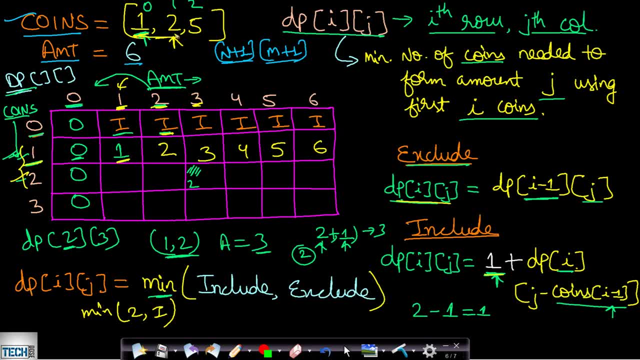 than our current denomination, which is 2. so whenever the current denomination is higher, then obviously we cannot include that coin, and so we will have to only exclude that coin. so if we exclude the current denomination, that is, the second denomination, then we will be having one less denomination and our amount to be found will be same. so we will be taking this number and we 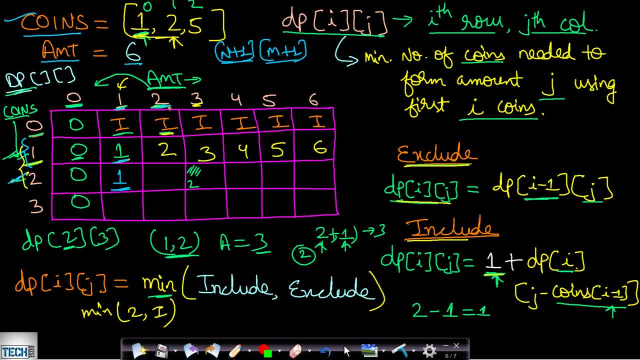 will just be copy pasting it now. this amount will be the minimum number of coins to form this amount. 2 is actually greater. therefore we will again compare two possibilities: include, exclude. if we exclude, then the value will come out to be two coins, and if we include, then this 2, that is this. 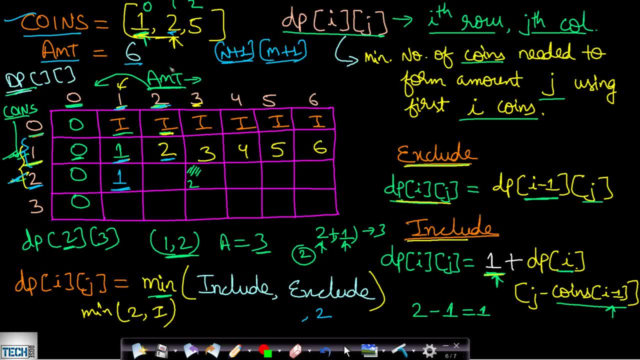 value 2 will get included and now, since we are including it, the new amount to be formed will be 2 minus the current value, which is 2, which will be 0. so we can form 0 by using 0 number of coins, so it will be 0 plus 1. 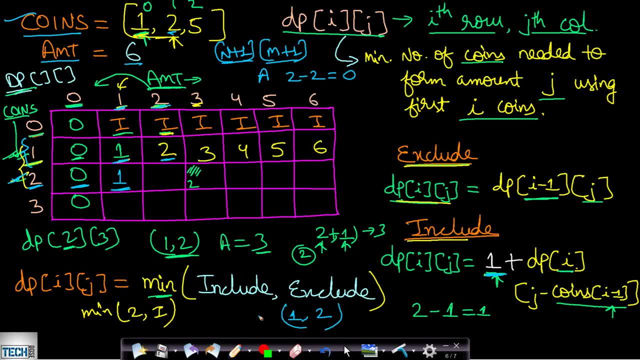 and that will come out to be 1. so the minimum of 1 comma 2 will be 1. therefore we can make amount equals to 2 by using 1 coin. I hope you understood this now for this 3. this 3 is greater than the. 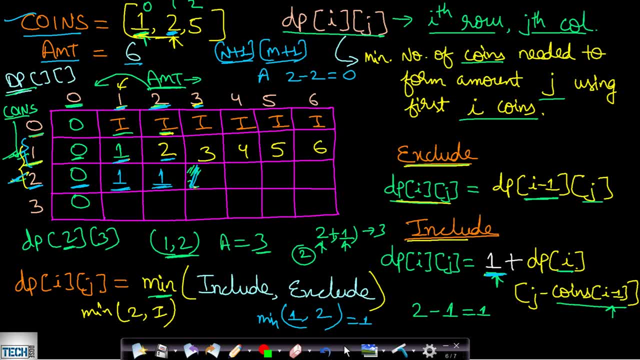 second denomination coin. so we will compare both the possibilities of inclusion and exclusion. if we exclude this, then it will be 3, and if we include this coin, 2, then this will be 1 plus 1, which will be 2, so 2 comma 3 will be 2. okay, so minimum number of coins to form this amount, 3 will be equals to 2. 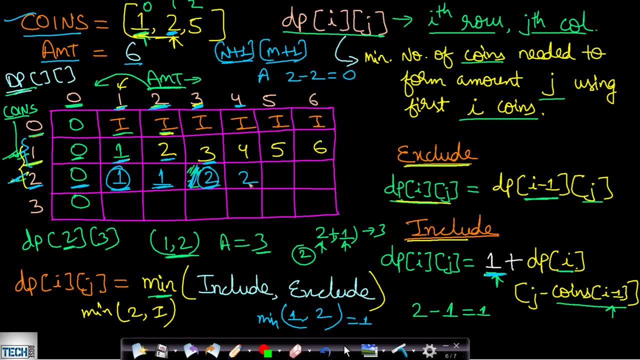 similarly for this 4, it will be 2, that is, this 1 plus 1. for this 5, it will be 3, which will be: uh, we will be including two number of points, 2 and then one number of 1.. now for this 6, it will be 3. 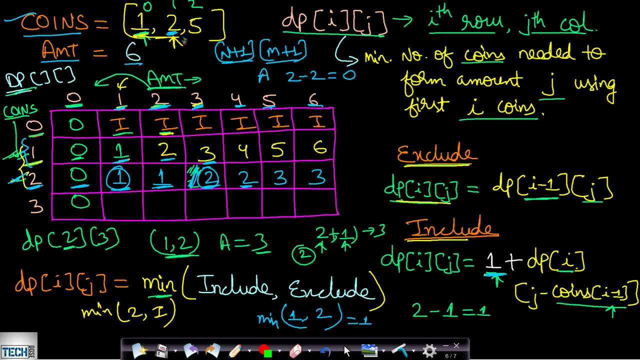 which will be this: 2 plus 1.. now, if we are having all these three denominations together, then this will be 5.. now, here this value is 5, and this 5 is actually greater than 1, 2, 3, 4.. so, for these amounts, 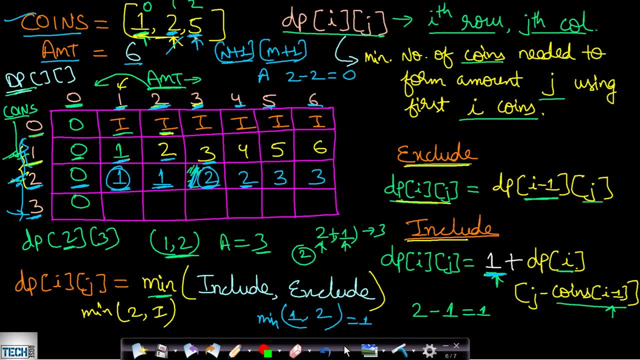 1, 2, 3, 4. we will actually not be able to include this 5.. so we will just be copying the top values. that means we will be just excluding the current denomination, which is 5.. so we will just copy these values here. now, this amount, 5, can be formed by using this element as well, so we 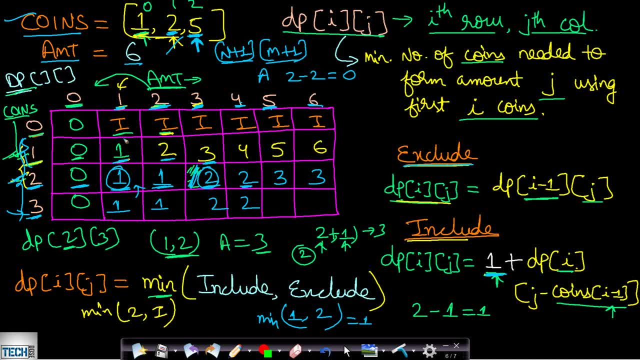 will be taking the minimum of two possibilities. we can either include this denomination 5.. so if we include this 5, then the amount to be found will be now 0, which is 5 plus 5. 0 can be found by using three denominations, by using zero number of coins. okay, so that will be 0 plus 1.. now we will 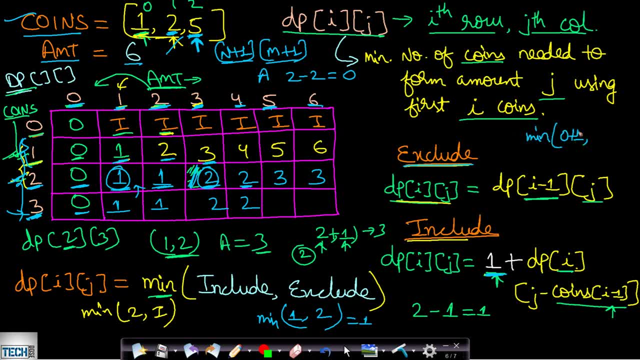 be taking minimum of 0 plus 1 comma. if we exclude this, then we can form it in three coins: 0 plus 1 comma, 3, which will be equals to 1.. so this will be 1.. now for this 6 as well. we will be making the choice between this inclusion. 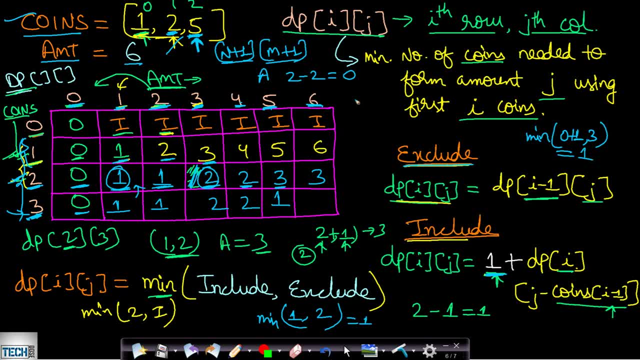 and exclusion. so if we include the current coin, then the new amount to be found will be the current denomination will get deducted from the amount value, then this will be 1.. so 1 can be formed by using three denominations using one coin. and since we have already included one coin, 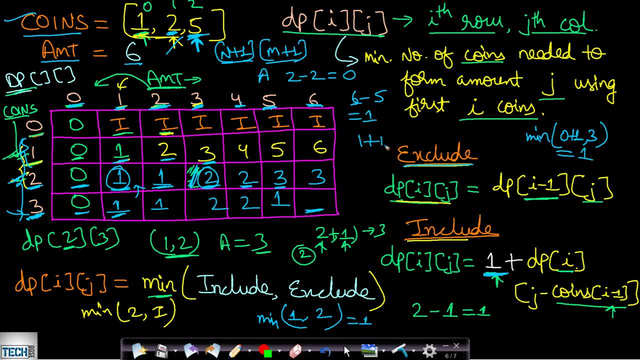 so the total number of coins in the inclusion case will be 1 plus 1, which will be 2. okay now the total number of coins for exclusion case is 3.. so the minimum of 2 comma 3 will be equals to 2.. so we will write here 2.. therefore the minimum number of coins which we can include. 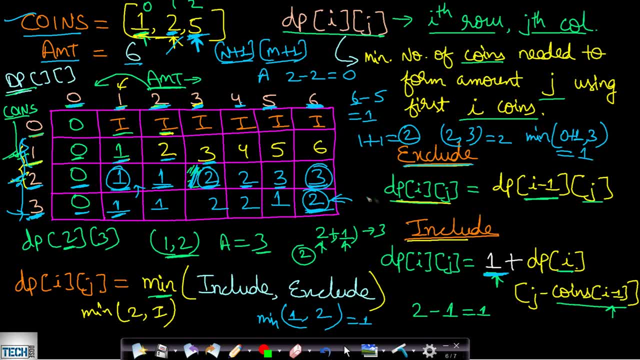 in order to form the sum, 6 will be equals to 2. and that will be nothing but 5 comma 1. okay, so this is the answer this last cell will be actually giving you if you are having all these denominations available. 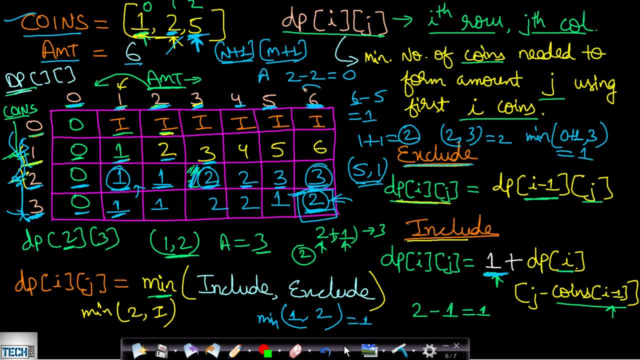 this combination can have infinite number of coins, and if the given amount to be formed is this one, which is 6 in this case, then the last cell will be giving you the minimum number of coins to form this amount. okay now, i hope you were able to understand this. so the time complexity. 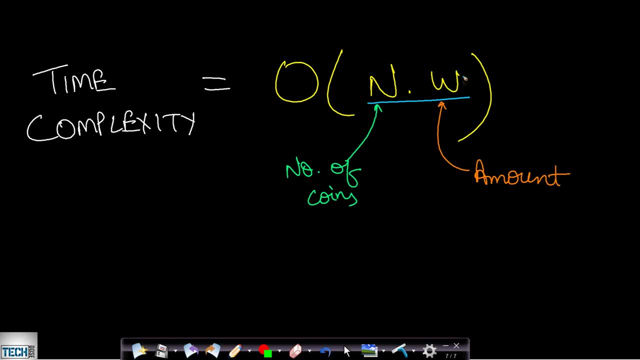 will be nothing but the size of the table, which is order of n into w, which is also the same as the knapsack problem. here, the n value is the number of coins and w is the amount. now let us look at the code. 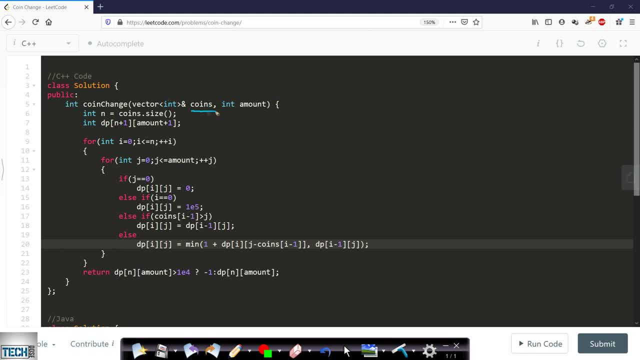 this is the code for the chain change problem. here we are given the coins as well as the amount. I have taken the number of coins in n and then I have taken the dp table. now this is the process of filling the dp table. 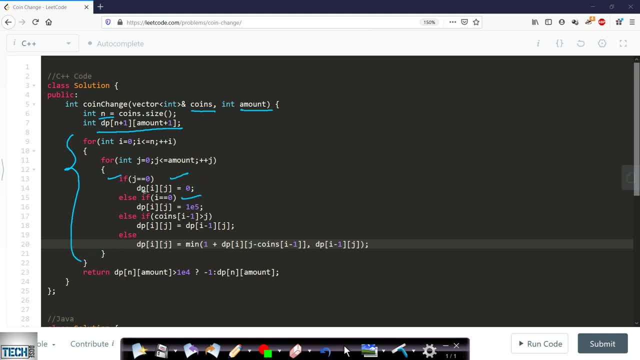 this is the boundary case. that means the first one is j equals to zero. that means, if amount value is equals to zero, then it will always be possible to form this amount value, which is zero, by using zero number of coins, by not including any coin. okay, otherwise. 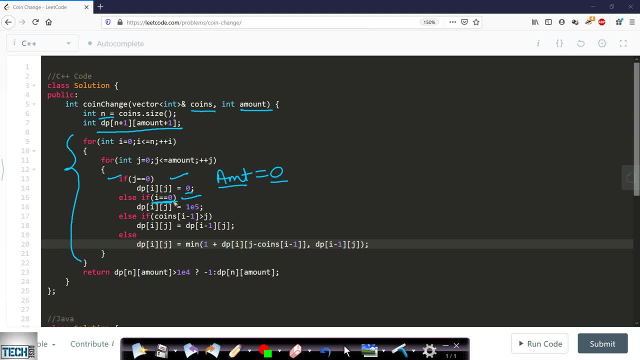 amount to be found is greater than zero and you are having zero number of coins, then it will never be possible to form that amount, and so we will be writing infinity here. here i have taken 10 to the power 5 as infinity. now, if these two boundary cases are not encountered and if the current 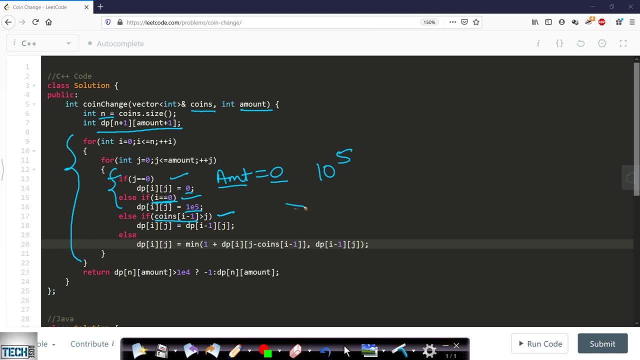 element, that is, the current denomination coin, is larger than the present amount to be found, then obviously we will not be able to include this coin, and so we will just take the exclusion case. that means we will go one level up and we will copy paste the solution. okay, otherwise, if we are, 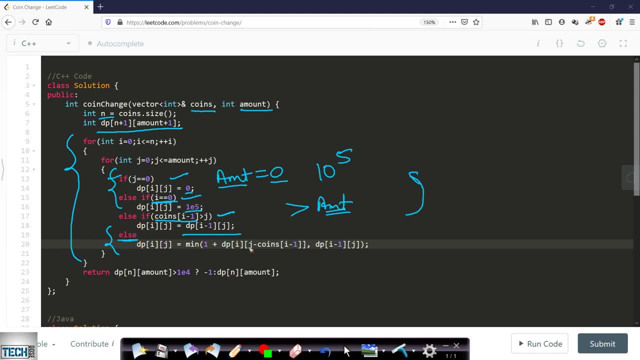 able to take the current denomination as well, then we will be taking the minimum of inclusion comma exclusion case, as i had shown you. so if we are including the current coin, then our number of coins will increase by one and we will remain in the same row. okay, because we are having the same. 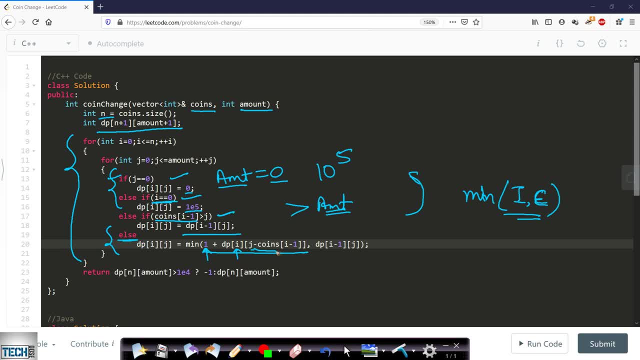 number of coins again. but the amount which we want to form now is not j, but it is j minus coins at i minus 1. so our total amount to be formed after including a coin which is coins at i minus 1 will get decremented okay. 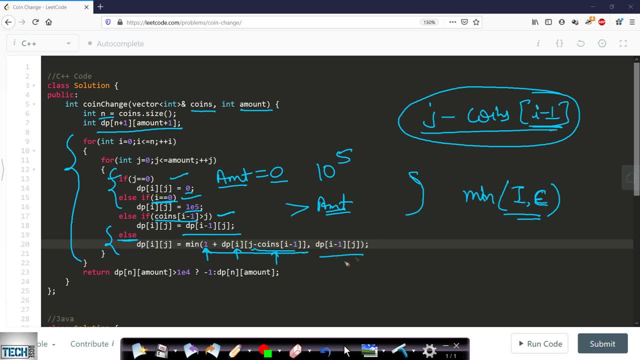 because we are including a coin. if we are excluding, then obviously we will just be going one level up and we will copy pasting. so we will be taking whichever is giving you the minimum number of coins to form that amount. so this is the entire logic for solving this problem and finally, we will check if the last